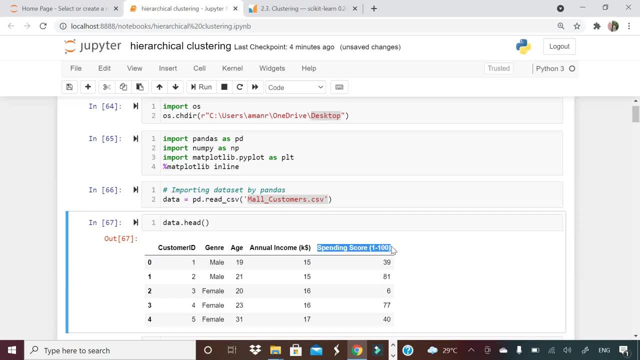 annual income of the customer and spending score of the customer. Okay, So these are the columns we have. Now we will try to run a hierarchical clustering on this particular data to see how clustered is looking like for the customers. Okay, Before that I want to subset. 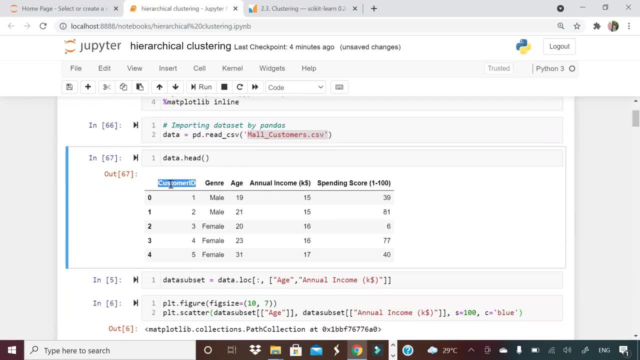 the data. Okay. So, as you can see, there are some categorical columns, for example this one, and customer ID is also kind of one kind of categorical, only you can say or identifier column, so not useful. So what I'm doing here is I'm just subsetting. 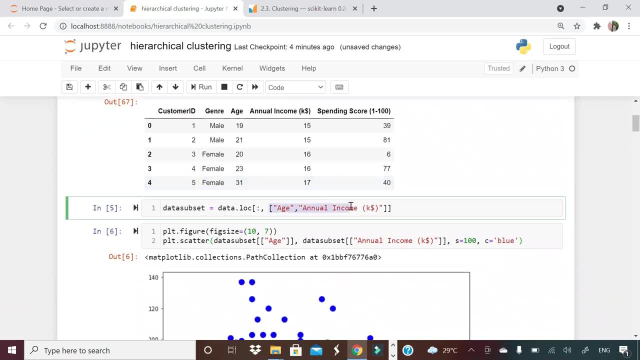 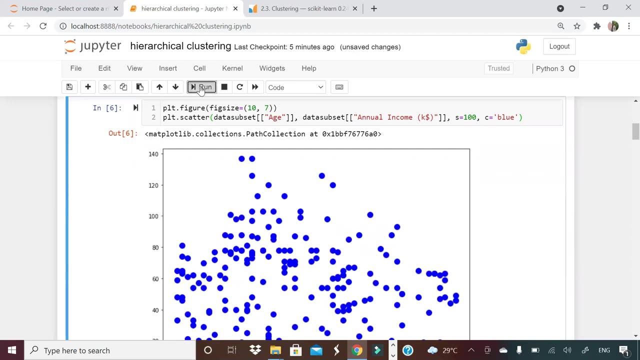 my data on two columns. one is age, another is an income. Okay, so I'm just taking two columns as an input to numerical columns. as an input, I'm creating a new data. I'm calling the data as data subset. okay, Let me run this And then I plot the data subset, guys. So once. 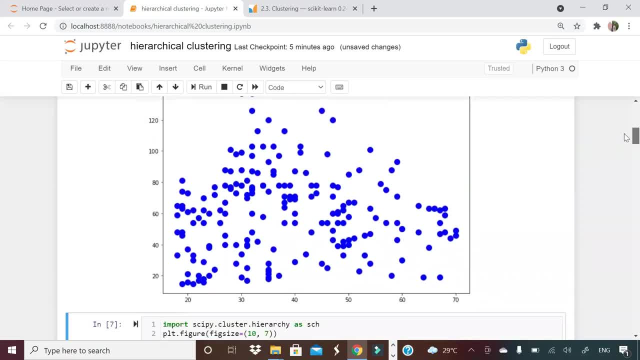 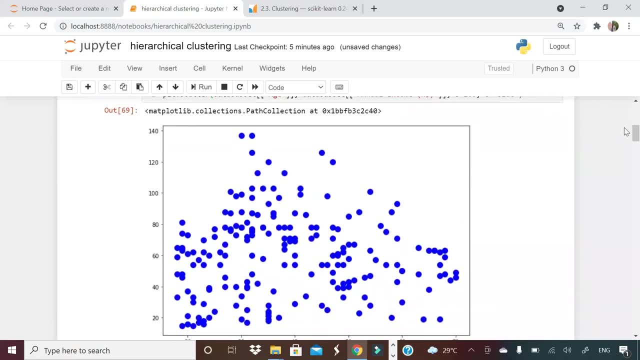 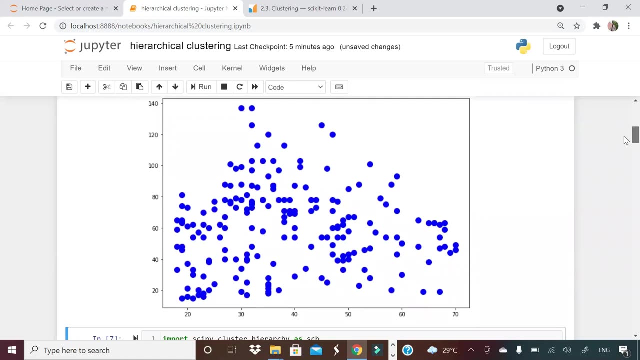 I plot this data subset: on x axis you have the age of the customers and on y axis you have the income of the customer, annual income of the customer. Okay so annual income ranges in the range of 0 to 140k and age ranges from 0 to 70, 75 k, 70, 75, that number. 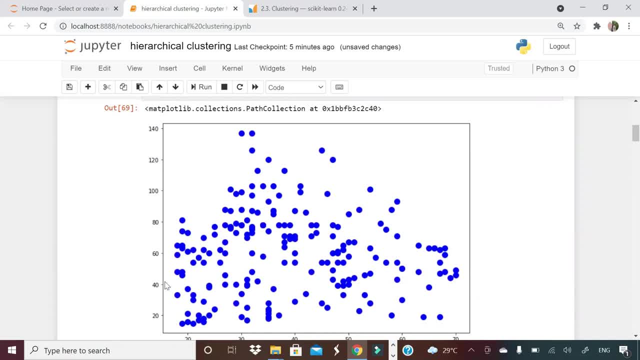 okay, now, if we see these data guys, then, uh, what do you think? will we be able to create some good cluster on this data? actually, there is no. uh, by looking, by looking at the data, by looking at this raw data, we can say that there is no such, you know, clustering kind of structure in this data. as 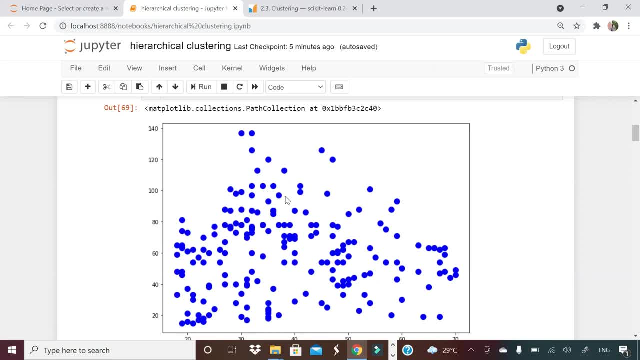 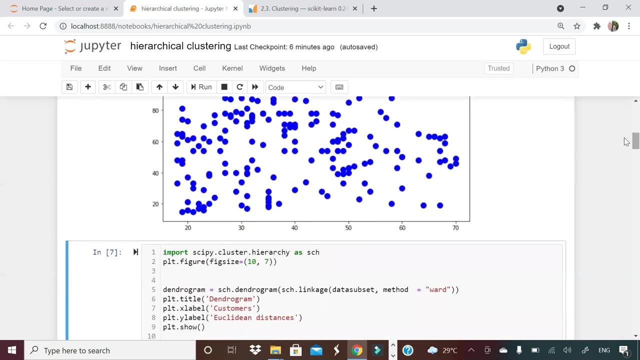 of now. okay, but still i will try to fit a heretical model and see how it is coming out, okay. so first of all, for heretical clustering, we need to know how many clusters we should have, right that we need to supply to know that what we do is we draw a dendrogram. so about this dendrogram i had 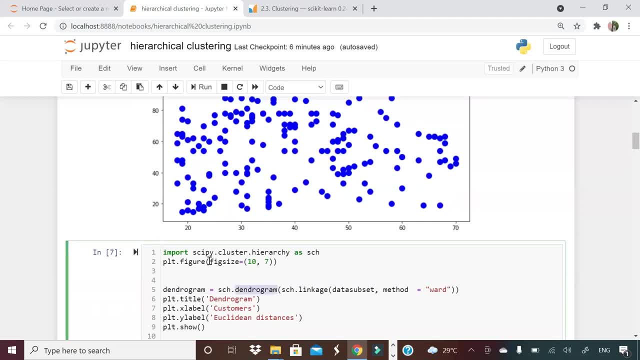 explained in my theoretical video, we draw a dendrogram like this. so if you see here from scipy cluster hierarchy, as sch dendrogram is equal to sch dot dendrogram, give your data. that is my data subset and method is equal to word. so methods i had explained in my last video, right? so method word i am giving here and if i run this, 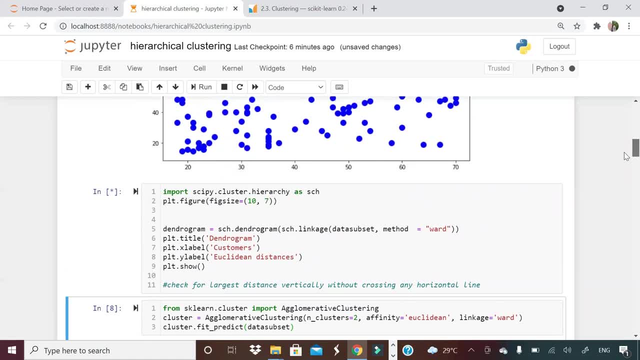 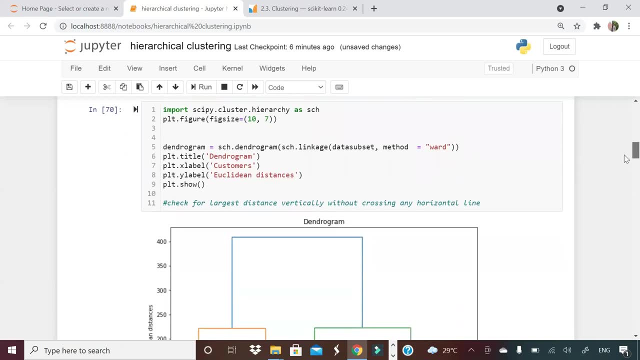 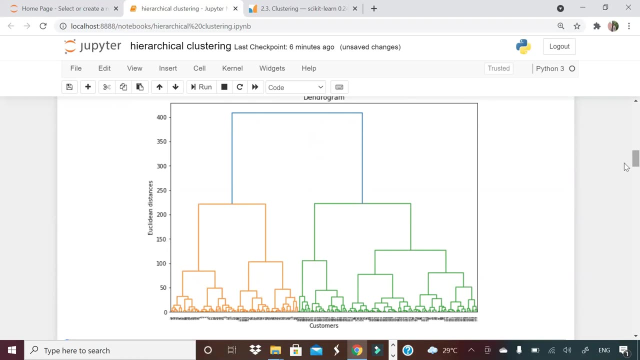 i will get a dendrogram like this. okay, dendrogram is plotting now, and once it comes i am going to tell you what to check in this dendrogram. okay, so here we have our dendrogram now. one thing to understand here, guys: you have to check the most lengthiest line vertically, or line with the most. 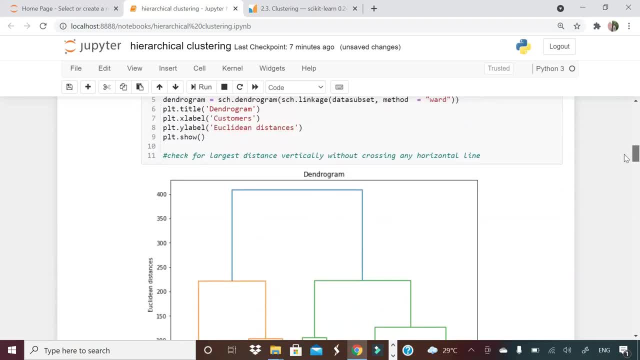 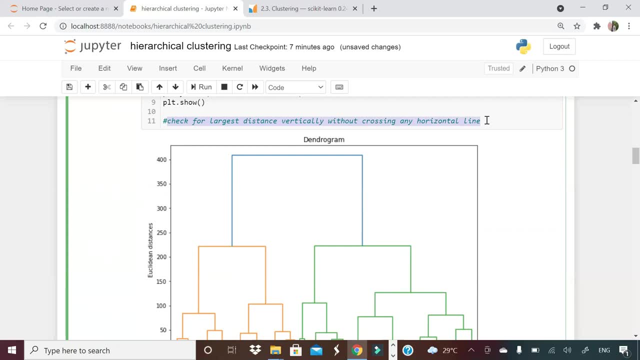 length without crossing any horizontal line. see, i have written here. check for the largest distance. now, here in this chart we are seeing this line and this line, two lines. okay, so both of these are more or less same length. only suppose, suppose there is one more line whose length comes up to. 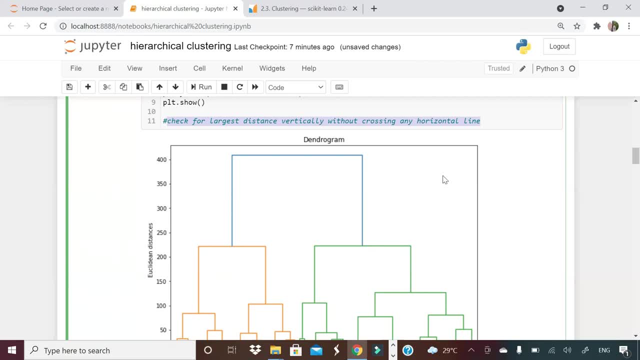 here, then that line will be the longest line, okay. and within that longest line, how many ever vertical line comes, that becomes your number of clusters, okay, i am repeating it again. see, you have a from the root, from the top, you have to see the longest blue line, okay. so in this case only two. 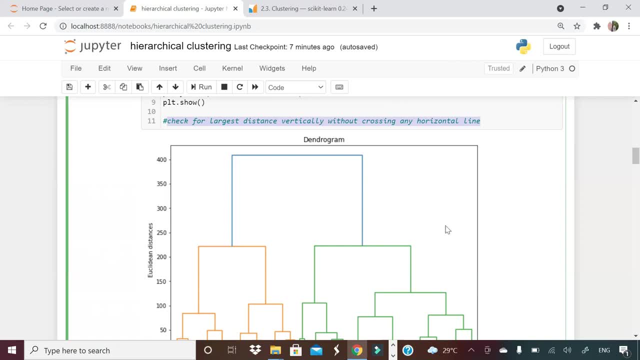 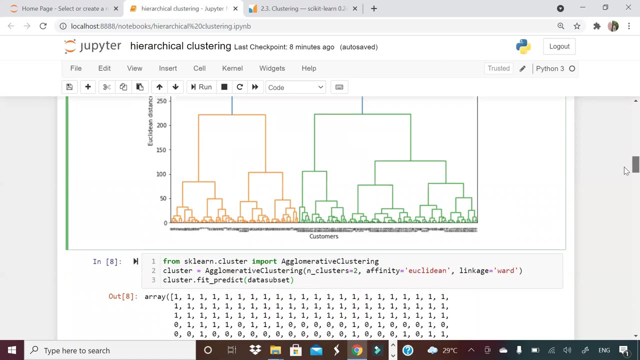 lines, so any one line can be longest. suppose there is one more line here like this. then you have to see how many lines equal to or smaller than this long line. that becomes your number of clusters. so here only two. so our number of clusters optimal is two. let's try running a heretical clustering. 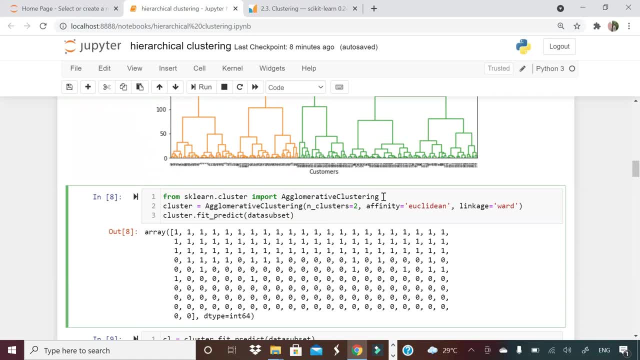 also known as agglomerative clustering. what i am doing here, i am importing from my skill and cluster agglomerative clustering. i am giving number of clusters, i am giving euclidean and i'm selling linkage is equal to what i am saying: cluster dot. fit underscore predict, which means fit on this data and then predict my clusters. 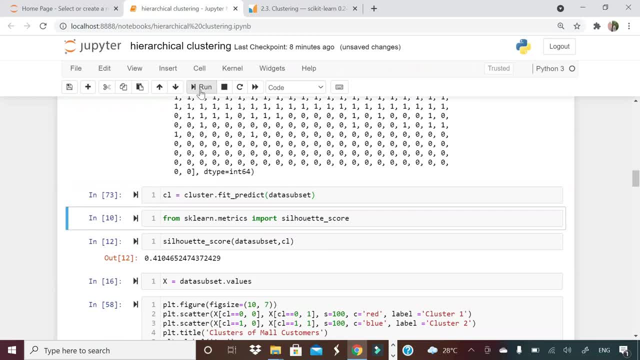 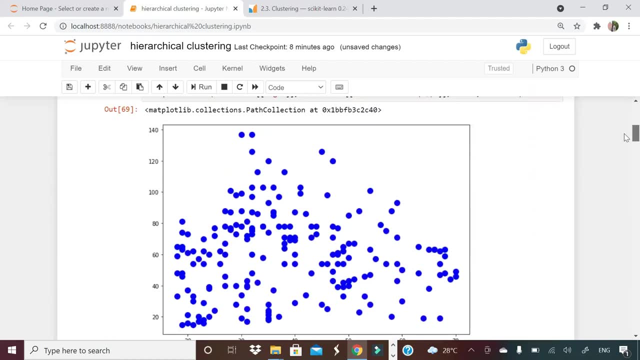 then i'm storing the prediction in a variable i am calling the silo test score, and the silo test score is very poor: 41. so, as we expected, guys, on this data, the cluster is not becoming good, the good clusters are not being formed. now, if you are watching this video, i am 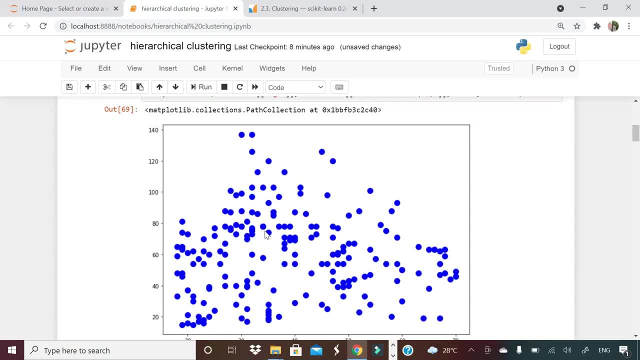 doing a mistake here. okay, so just think if you can find out what mistake i'm doing, one basic mistake i'm doing- okay. but i will discuss about that in the end, but first i will try some other clustering model on this. okay, so let us try db scan and let us try k means also to see how it is coming, okay. 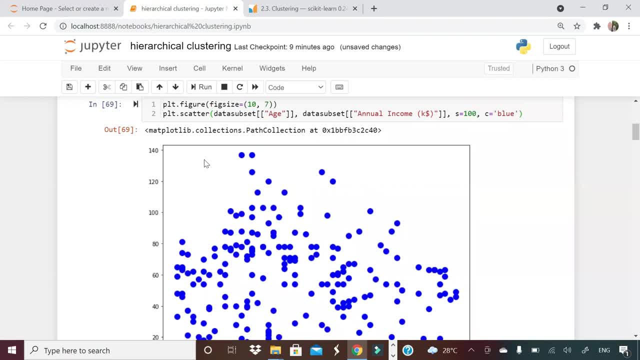 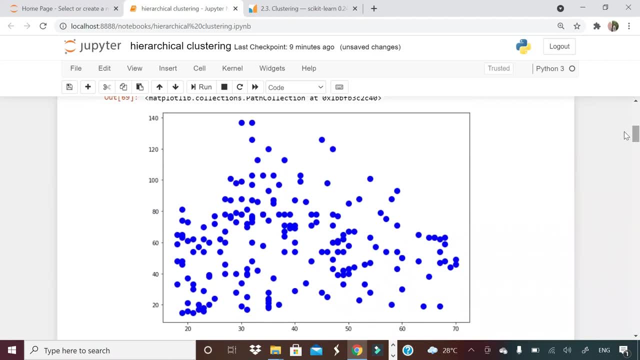 now looking at the data structure guys, what do you think db scan will do? good or will not do good? the reason i am discussing these topics is this is a workshop kind of video guys. so you should look at the data and you should try to figure out. uh, you should think how k means work. you should think how dbs can work. 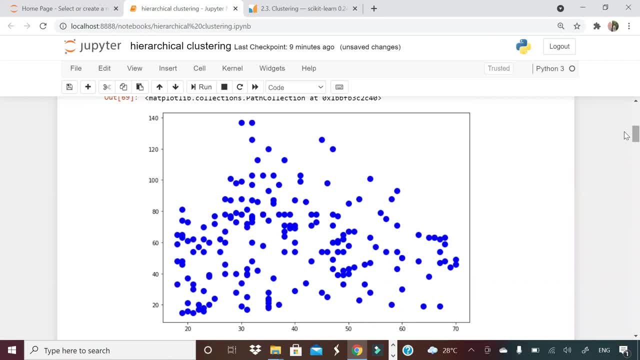 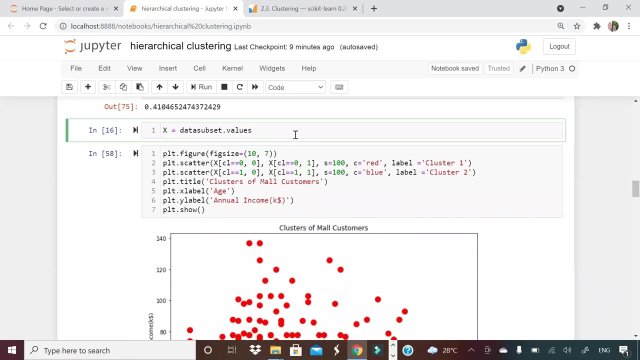 and then you should be able to figure out whether that will give a good result or not good result. so here, do you have density like data? i think no. let us see how db scan does here, okay. so here do you have density like data? i think no. let us see how db scan does here, okay. so if we come here, 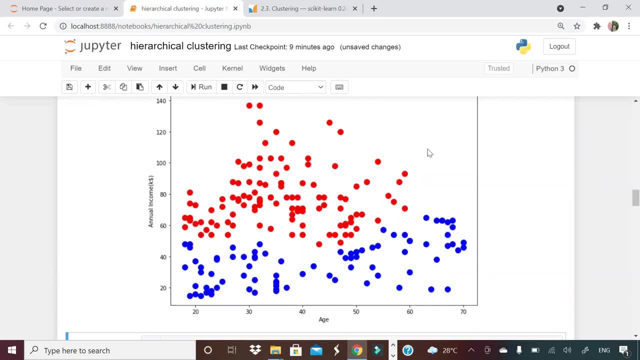 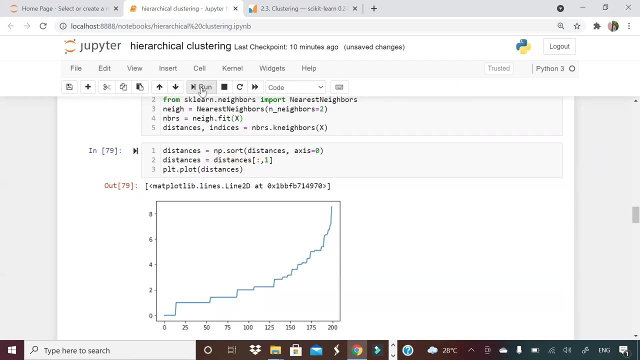 i am just plotting from the ever created charts, ever created agglomerative clustering. i am plotting the clusters. so this is how the clusters are formed. okay, here another hint. what mistake i am doing. okay, now let us move forward and run a db scan clustering. so same way i am printing and 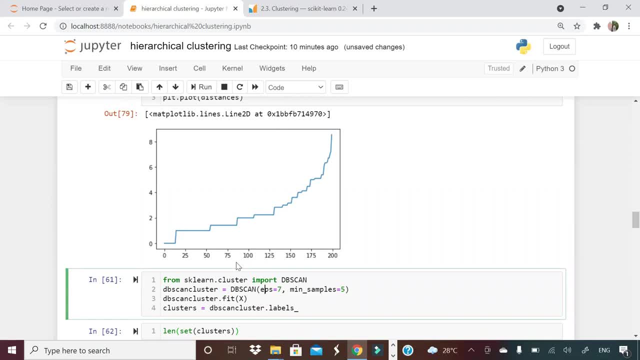 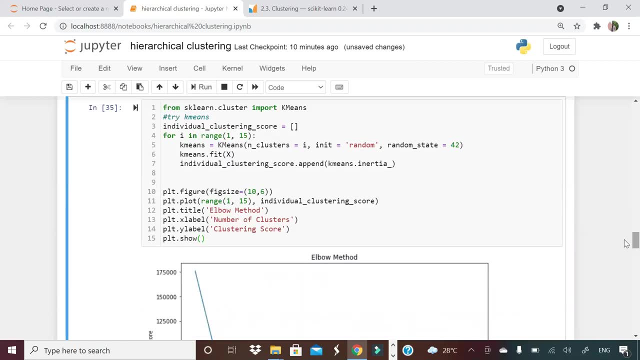 example from here, let's say five or seven I can give. I have given seven here. I am trying to run a DB scan cluster. I get three cluster and I get C lot A of how much, 28,, which is very. 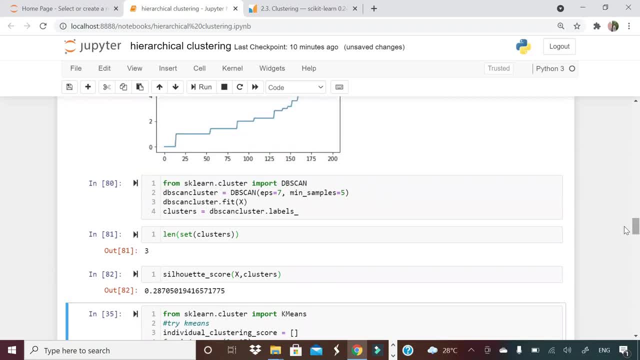 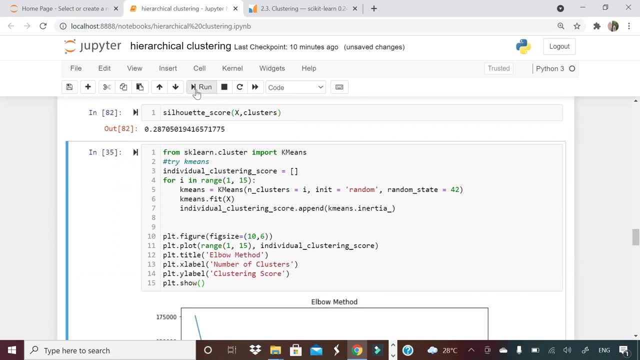 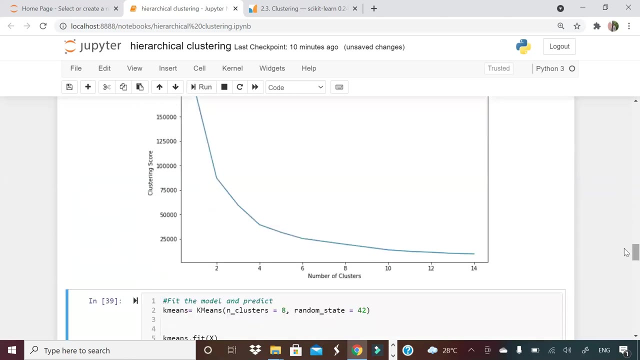 very poor, poor than previous one, also poor than your hierarchical clustering. also, Let us try. K means now Okay. so for K means I want to know the optimal number of clusters. hence I'm plotting elbow. If I'm plotting elbow, then elbow comes like this: From this elbow I take either four. 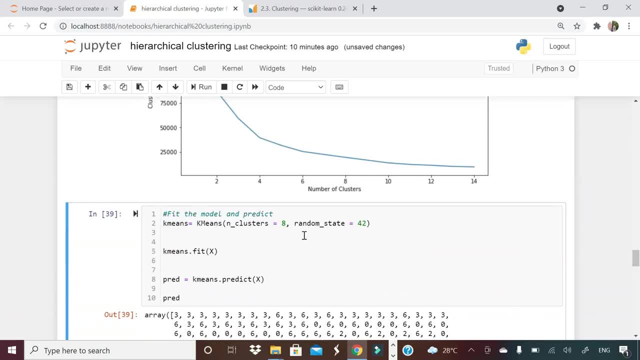 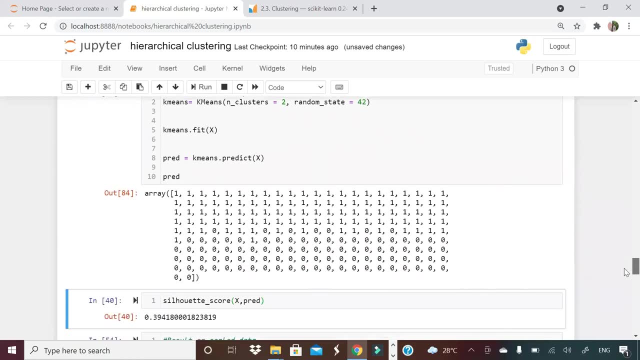 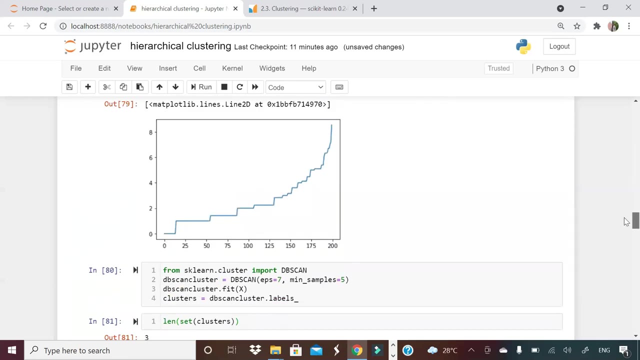 or two or something. In this case I have taken eight because I was running many attritions. For example, if I take two, then two clusters I'm getting Okay, and the C lot A of 42 I'm getting, which is still poor. Now coming to the answer of what mistake I was doing: okay, all the three. 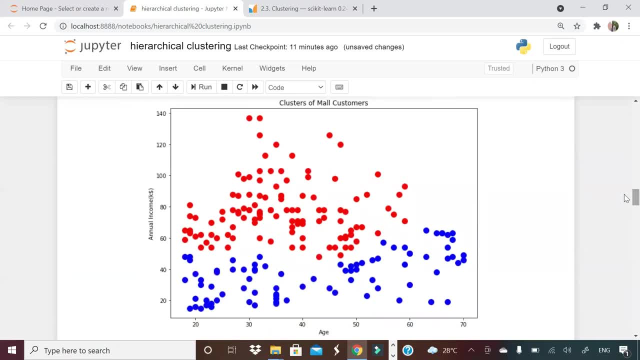 algorithms we have run and we are not getting good result. So, if you can see, guys, age and income are on different scales, right? So age is in the range of 0 to 100, whereas income is in the range of 140k, 120k, like that. So what we should do, we should normalize. 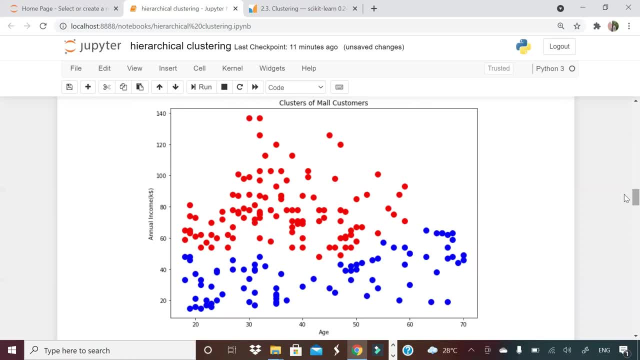 this data because all the clustering algorithm, apart from DB scan- DB scan also- all the clustering algorithm uses distances, that is, Euclidean distance or any other distance. So we need to normalize And that is what I'm doing here. I'm saying: 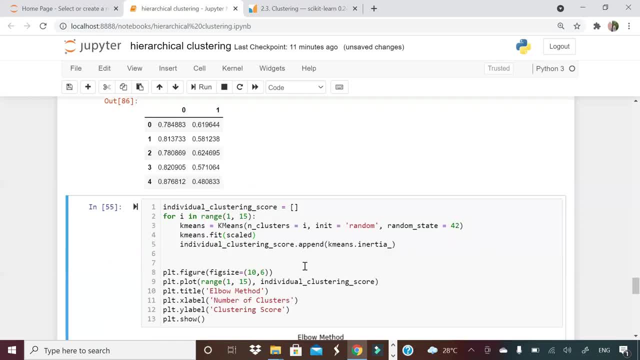 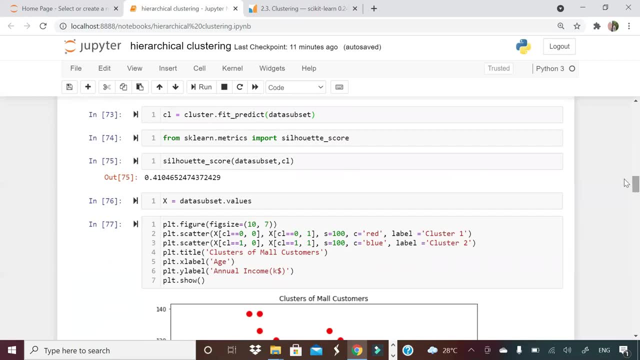 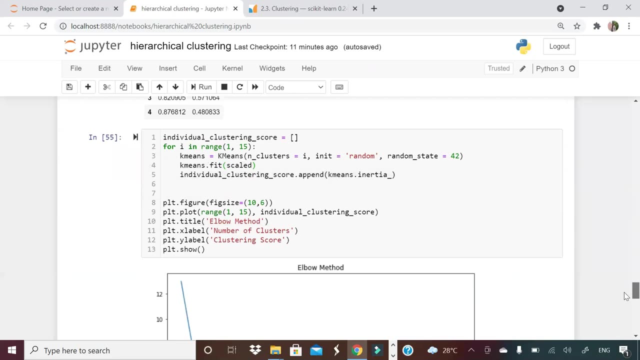 from a skill and pre-processing: import, normalize. I'm normalizing my x. x is nothing but your values. If you see here, x is nothing but your data. on which clusters are being formed here, data subset, dot values. Okay, So I'm just normalizing x And one more time I'm running. 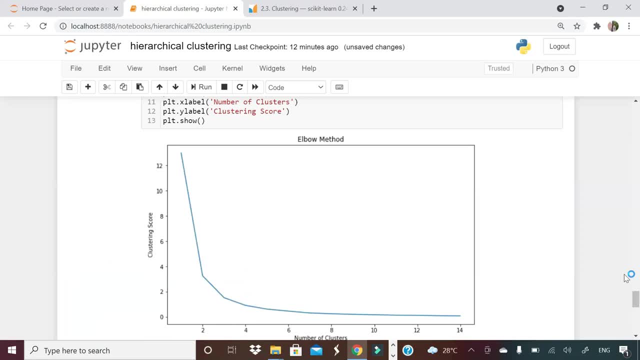 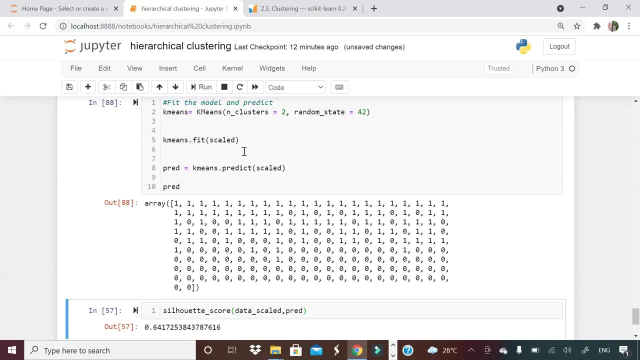 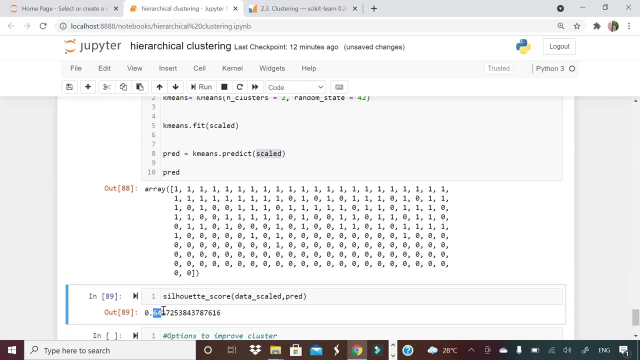 my optimal number of cluster code, And here I'm getting this kind of chart. So I will try with two. one more time on my scaled data, If you see here on my scale data, okay, And then I'm getting a serota of 64%. So by doing a small thing, guys, 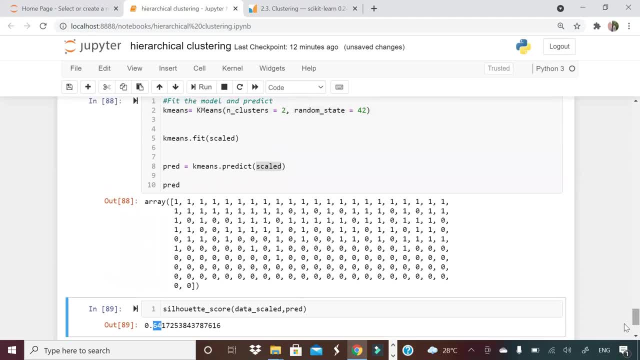 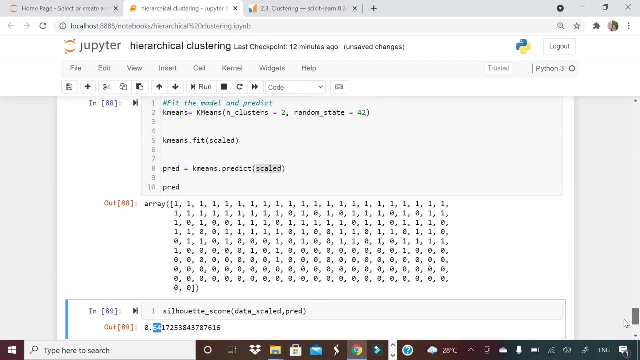 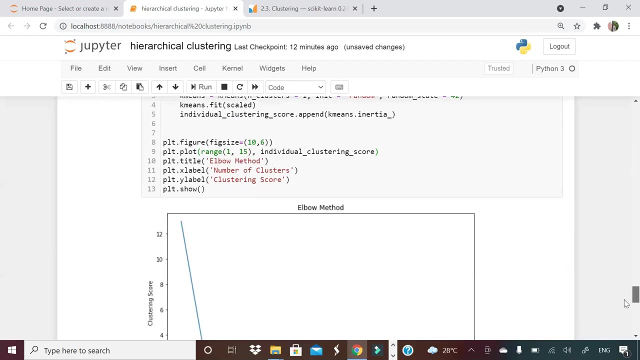 by that, by just scaling on the data, same variable, everything, I'm able to improve my model significantly, Okay. So this exercise was to show you what kind of mistakes we make in clustering, Okay, And how it can hamper your cluster badly. Now I want to discuss two things here. One is: 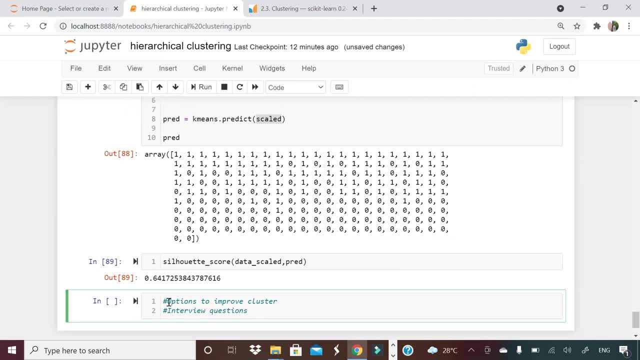 how else you can improve your model. So options, how to improve cluster Few things that come to my mind straight away is: if we have some more dimensions, if we have some more data points, then maybe model will be able to learn some patterns. 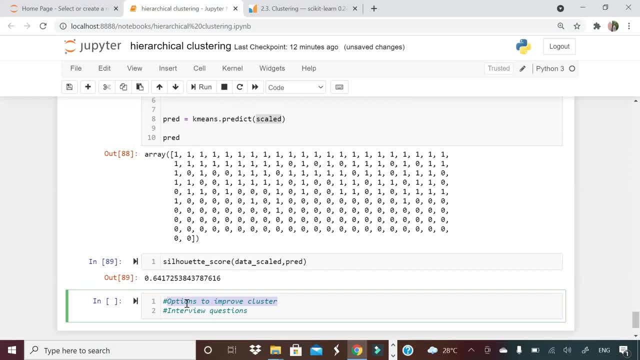 maybe we can do some bit of PCA, we can do some bit of other other feature engineering which will help model create. better cluster probably, but definitely more number of variables and more number of records will help here. Okay, So that is what my view. 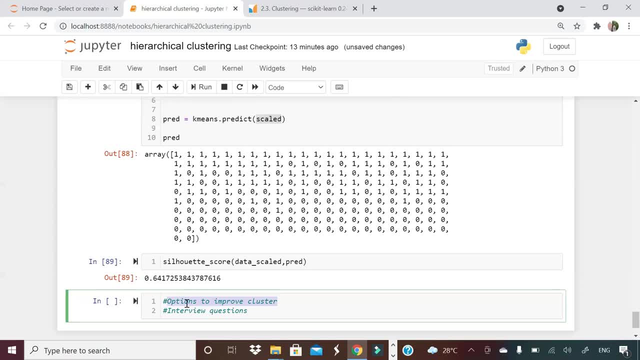 I want you to write in How we can improve. I will upload this notebook in my drive. you can take and you can start working on this. Okay, And then interview questions. So whole idea of all my seven, eight videos that I